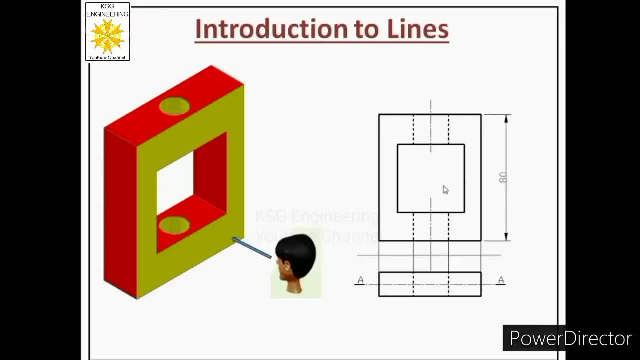 Let us say these are its front view and top views. Now, in these two views, different types of lines are used. Each line has a specific meaning. Each line has a specific function. So in this lecture, we will learn about different types of lines commonly used in engineering drawing. 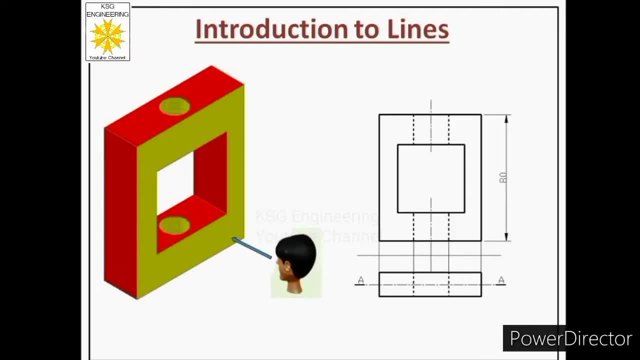 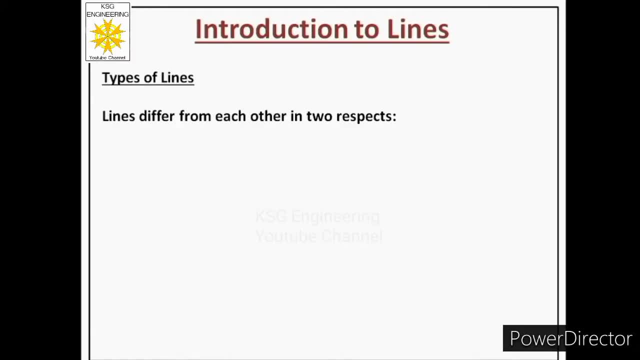 We will learn about their name, construction and application. First of all, we will discuss how lines differ from each other. Lines differ from each other in two respects. First, based on their thickness or weight. So, based on this category, we define lines. 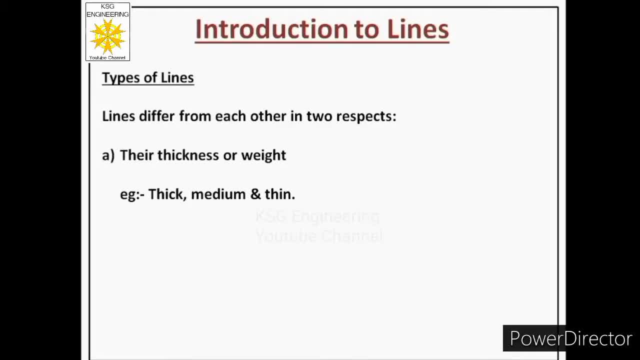 So, based on this category, we define lines. So, based on this category, we define lines. We define lines as thick lines, medium lines and thin lines. We define lines as thick lines, medium lines and thin lines. We define lines as thick lines, medium lines and thin lines. 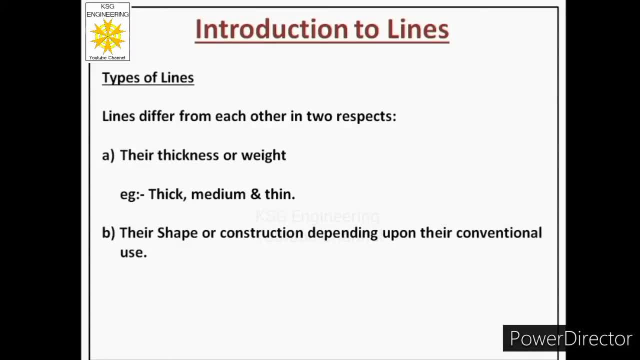 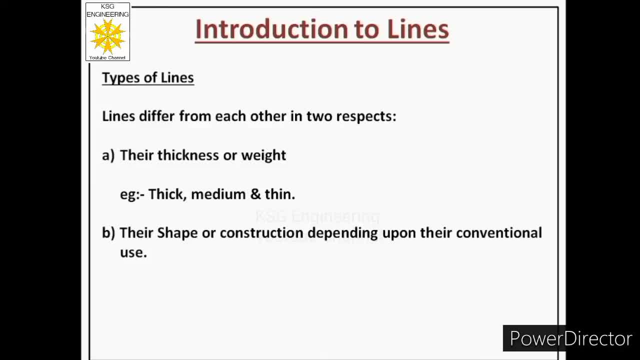 The second point of difference between any two lines is based on their shape or construction, depending upon their conventional use. The second point of difference between any two lines is based on their shape or construction, depending upon their conventional use. So let us discuss these two in detail. 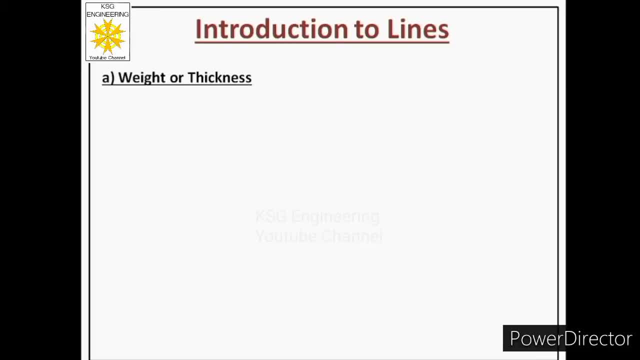 So let us discuss these two in detail. First we will discuss about weight or thickness. First we will discuss about weight or thickness. So let me draw two lines. So let me draw two lines. Now, if we have to compare these two lines, then we can say that this is a thick line and this is a thin line. 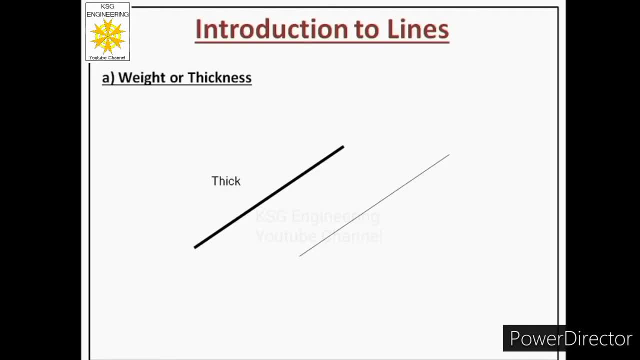 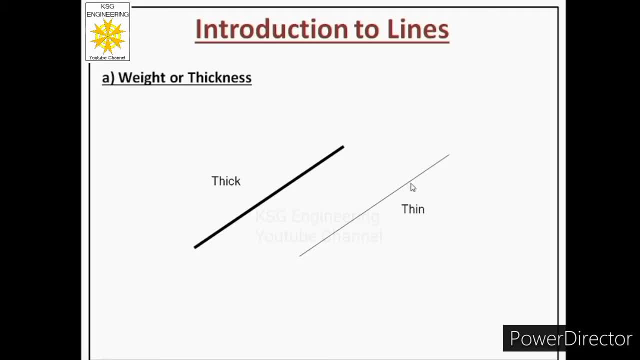 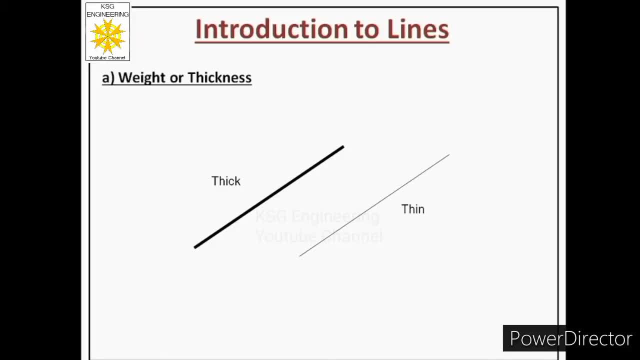 So we have differentiated these two lines based on their weight or thickness. So we have differentiated these two lines based on their weight or thickness. So we have differentiated these two lines based on their weight or thickness. So in engineering drawing, we have three types of lines: based on their thickness or weight. 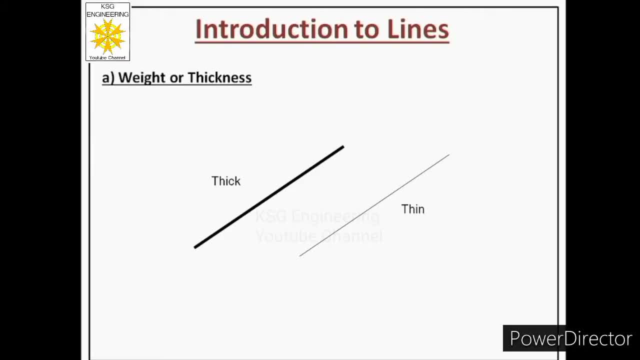 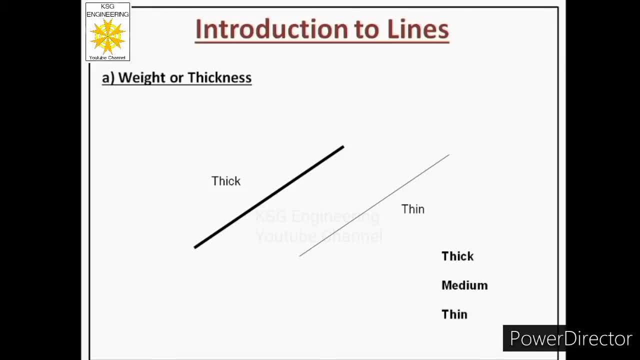 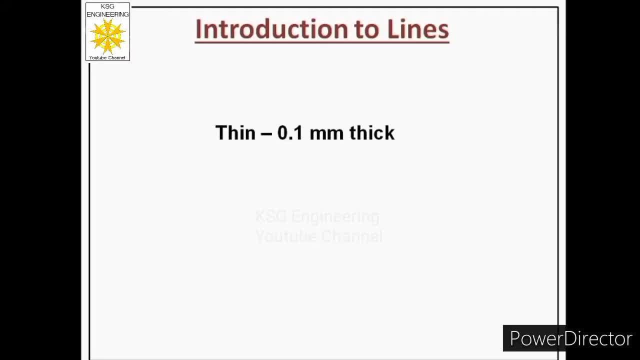 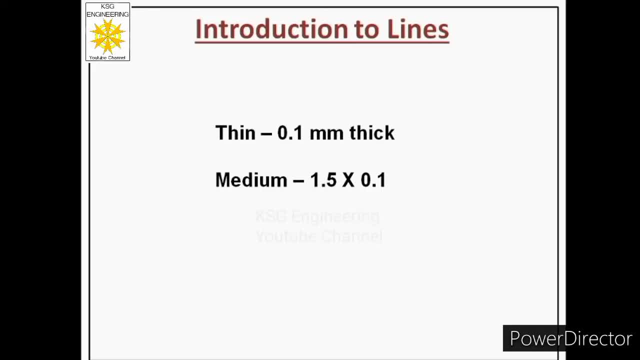 Then we have to take thickness of medium line as 1.5 times the thickness of thin line. Then we have to take thickness of medium line as 1.5 times the thickness of thin line. Then we have to take thickness of medium line as 1.5 times the thickness of thin line. 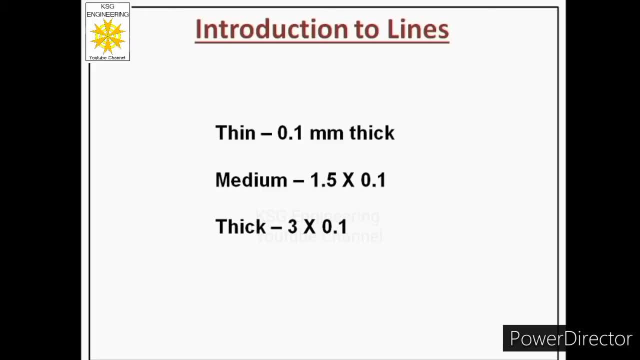 Similarly, if we want to draw a thick line, then we have to take thickness of thick line 3 times the thickness of thin line taken by us. Similarly, if we want to draw a thick line, then we have to take thickness of thick line 3 times the thickness of thin line taken by us. 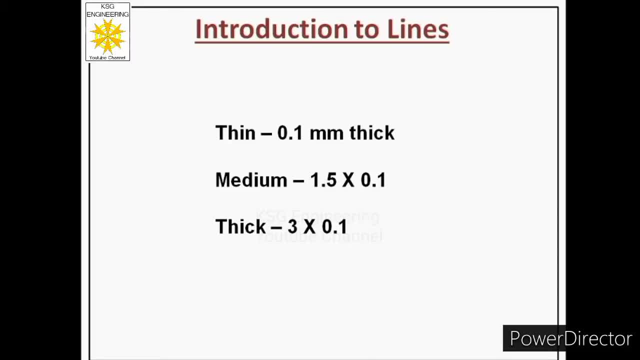 Similarly, if we want to draw a thick line, then we have to take thickness of thick line 3 times the thickness of thin line taken by us. Similarly, if we want to draw a thick line, then we have to take thickness of thick line 3 times the thickness of thin line taken by us. 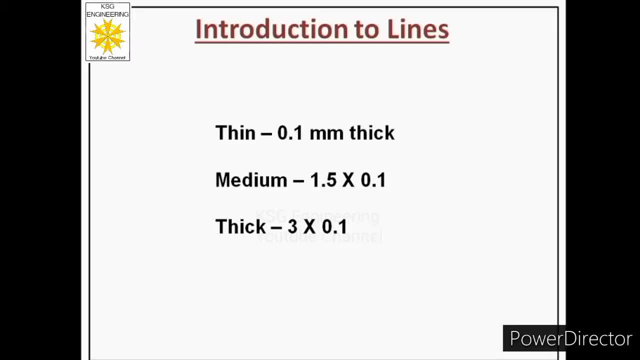 Similarly, if we want to draw a thick line, then we have to take thickness of thin line 3 times the thickness of thin line taken by us. Similarly, if we want to draw a thick line, then we have to take thickness of thin line 3 times the thickness of thin line taken by us. 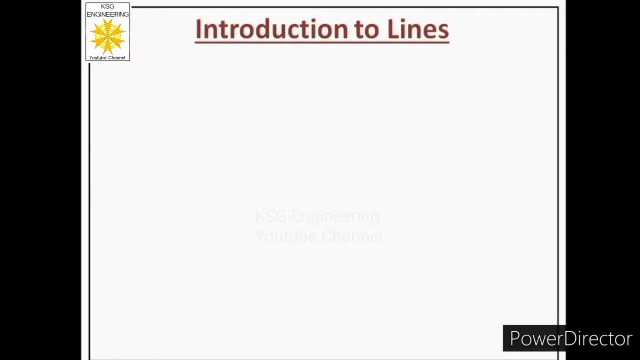 Similarly, if we want to draw a thick line, then we have to take thickness of thin line 3 times the thickness of thin line taken by us. Similarly, if we want to draw a thick line, then we have to take thickness of thin line 3 times the thickness of thin line taken by us. 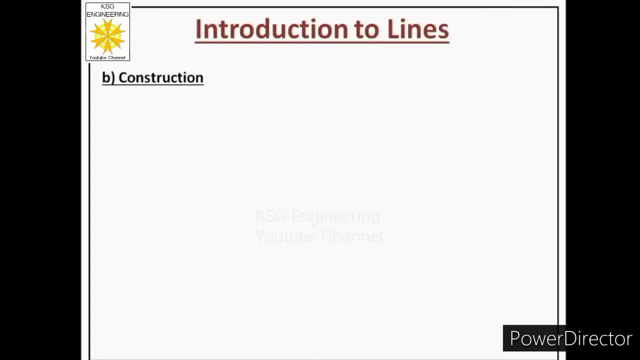 Similarly, if we want to draw a thick line, then we have to take thickness of thin line 3 times the thickness of thin line taken by us. Similarly, if we want to draw a thick line, then we have to take thickness of thin line 3 times the thickness of thin line taken by us. 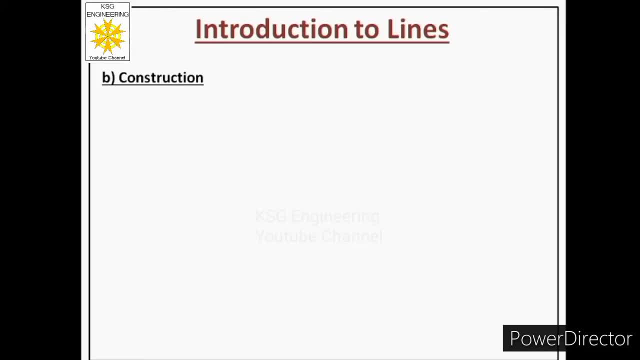 Similarly, if we want to draw a thick line, then we have to take thickness of thin line 3 times the thickness of thin line taken by us. Similarly, if we want to draw a thick line, then we have to take thickness of thin line 3 times the thickness of thin line taken by us. 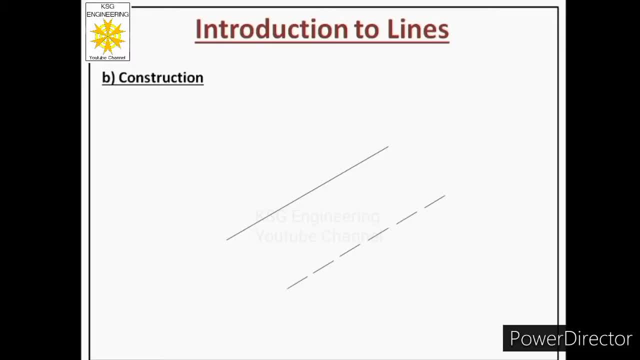 Similarly, if we want to draw a thick line, then we have to take thickness of thin line 3 times the thickness of thin line taken by us. Similarly, if we want to draw a thick line, then we have to take thickness of thin line 3 times the thickness of thin line taken by us. 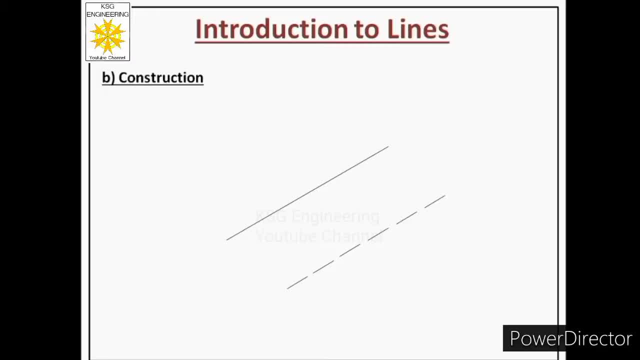 Similarly, if we want to draw a thick line, then we have to take thickness of thin line 3 times the thickness of thin line taken by us. Similarly, if we want to draw a thick line, then we have to take thickness of thin line 3 times the thickness of thin line taken by us. 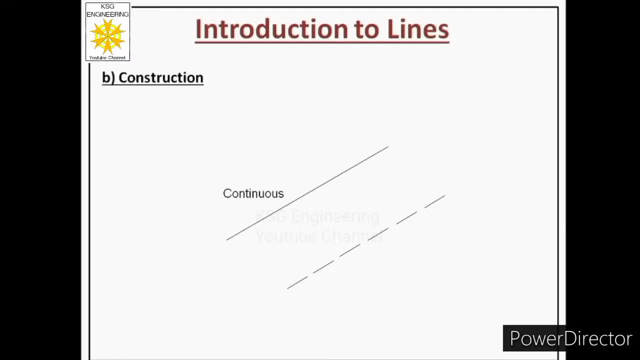 Similarly, if we want to draw a thick line, then we have to take thickness of thin line 3 times the thickness of thin line taken by us. Similarly, if we want to draw a thick line, then we have to take thickness of thin line 3 times the thickness of thin line taken by us. 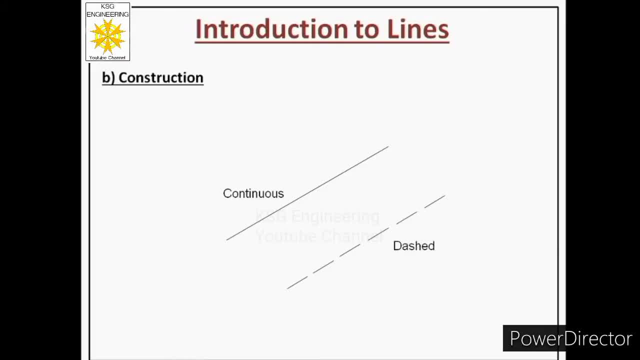 Similarly, if we want to draw a thick line, then we have to take thickness of thin line 3 times the thickness of thin line taken by us. Similarly, if we want to draw a thick line, then we have to take thickness of thin line 3 times the thickness of thin line taken by us. 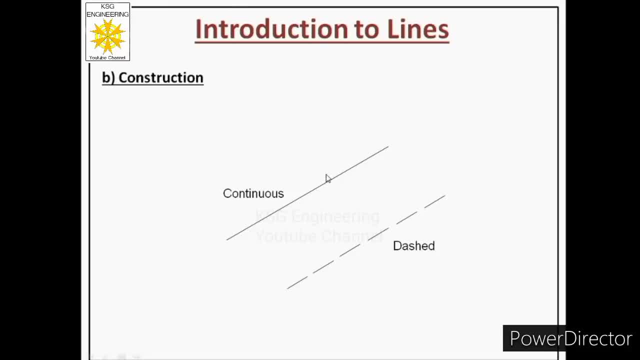 Similarly, if we want to draw a thick line, then we have to take thickness of thin line 3 times the thickness of thin line taken by us. Similarly, if we want to draw a thick line, then we have to take thickness of thin line 3 times the thickness of thin line taken by us. 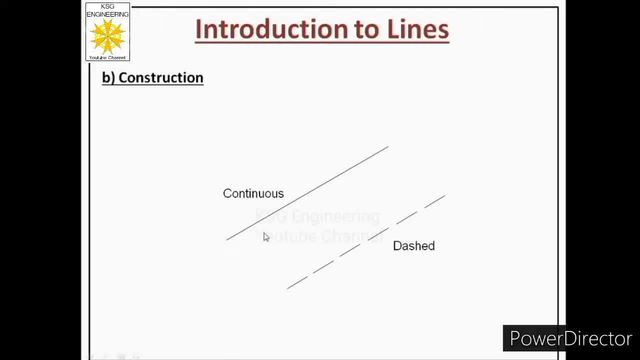 Similarly, if we want to draw a thick line, then we have to take thickness of thin line 3 times the thickness of thin line taken by us. Similarly, if we want to draw a thick line, then we have to take thickness of thin line 3 times the thickness of thin line taken by us. 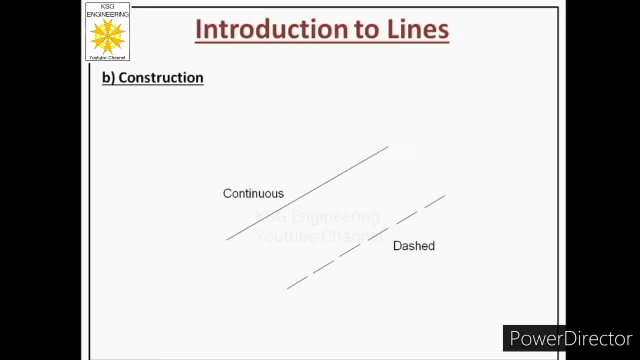 Similarly, if we want to draw a thick line, then we have to take thickness of thin line 3 times the thickness of thin line taken by us. Similarly, if we want to draw a thick line, then we have to take thickness of thin line 3 times the thickness of thin line taken by us. 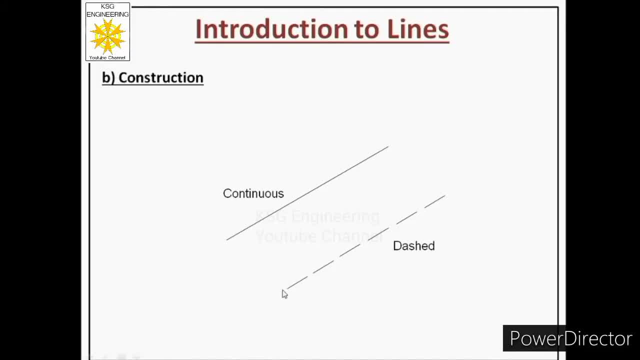 Similarly, if we want to draw a thick line, then we have to take thickness of thin line 3 times the thickness of thin line taken by us. Similarly, if we want to draw a thick line, then we have to take thickness of thin line 3 times the thickness of thin line taken by us. 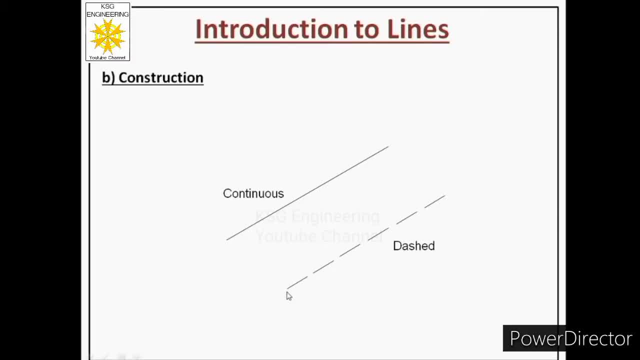 Similarly, if we want to draw a thick line, then we have to take thickness of thin line 3 times the thickness of thin line taken by us. Similarly, if we want to draw a thick line, then we have to take thickness of thin line 3 times the thickness of thin line taken by us. 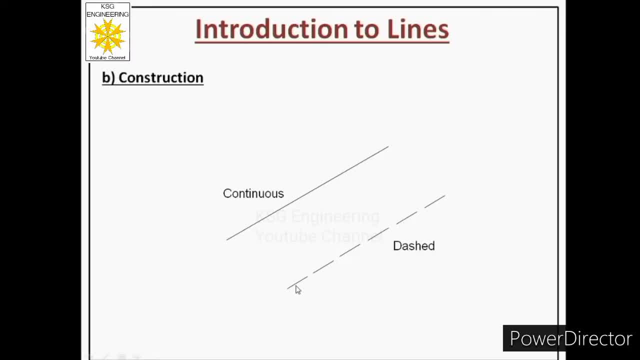 Similarly, if we want to draw a thick line, then we have to take thickness of thin line 3 times the thickness of thin line taken by us. Similarly, if we want to draw a thick line, then we have to take thickness of thin line 3 times the thickness of thin line taken by us. 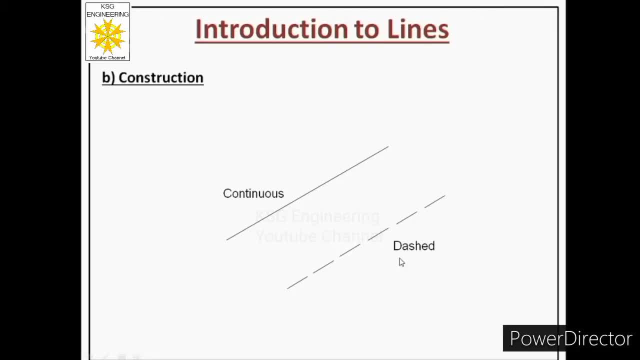 Similarly, if we want to draw a thick line, then we have to take thickness of thin line 3 times the thickness of thin line taken by us. Similarly, if we want to draw a thick line, then we have to take thickness of thin line 3 times the thickness of thin line taken by us. 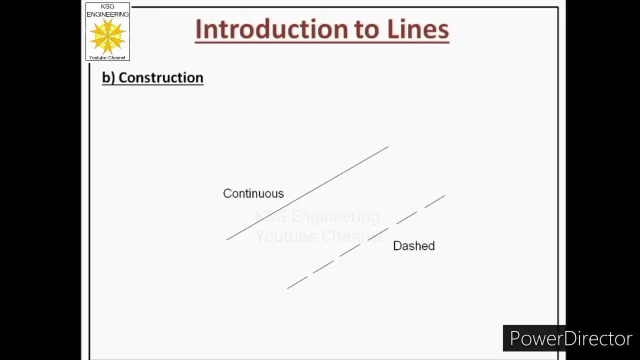 Similarly, if we want to draw a thick line, then we have to take thickness of thin line 3 times the thickness of thin line taken by us. Similarly, if we want to draw a thick line, then we have to take thickness of thin line 3 times the thickness of thin line taken by us. 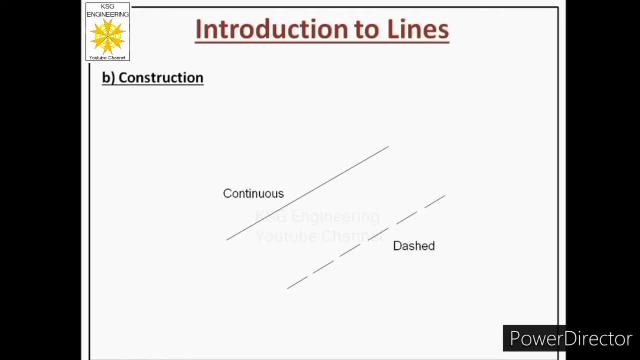 Similarly, if we want to draw a thick line, then we have to take thickness of thin line 3 times the thickness of thin line taken by us. Similarly, if we want to draw a thick line, then we have to take thickness of thin line 3 times the thickness of thin line taken by us. 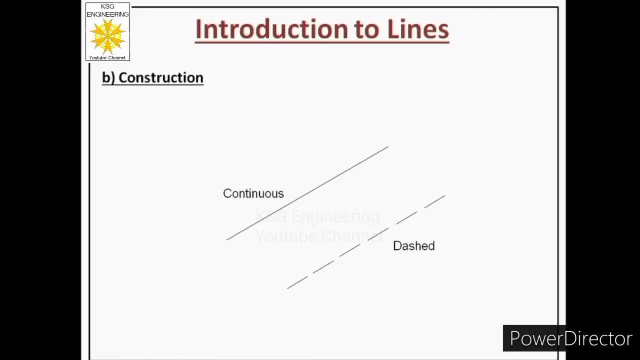 Similarly, if we want to draw a thick line, then we have to take thickness of thin line 3 times the thickness of thin line taken by us. Similarly, if we want to draw a thick line, then we have to take thickness of thin line 3 times the thickness of thin line taken by us. 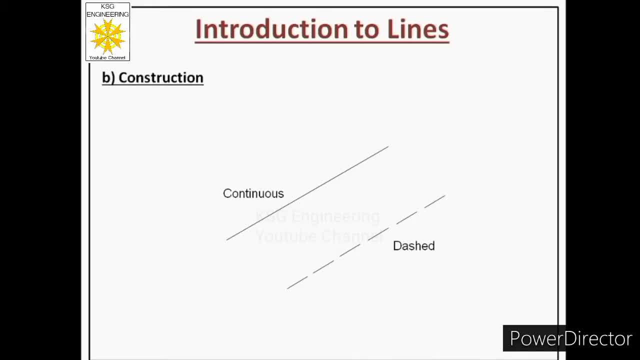 Similarly, if we want to draw a thick line, then we have to take thickness of thin line 3 times the thickness of thin line taken by us. Similarly, if we want to draw a thick line, then we have to take thickness of thin line 3 times the thickness of thin line taken by us. 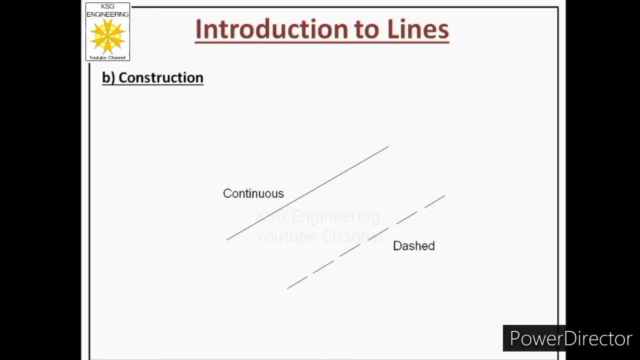 Similarly, if we want to draw a thick line, then we have to take thickness of thin line 3 times the thickness of thin line taken by us. Similarly, if we want to draw a thick line, then we have to take thickness of thin line 3 times the thickness of thin line taken by us. 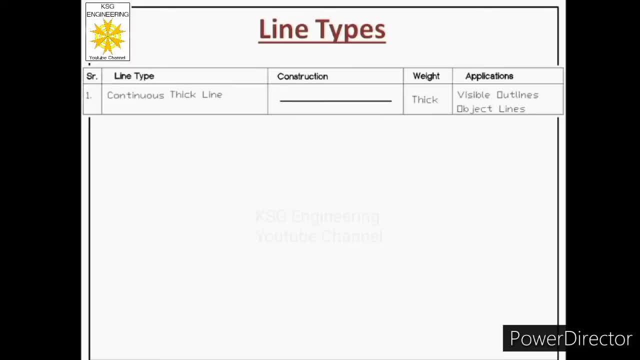 Similarly, if we want to draw a thick line, then we have to take thickness of thin line 3 times the thickness of thin line taken by us. Similarly, if we want to draw a thick line, then we have to take thickness of thin line 3 times the thickness of thin line taken by us. 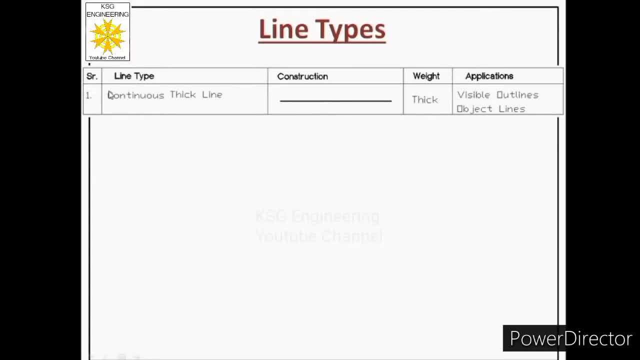 Similarly, if we want to draw a thick line, then we have to take thickness of thin line 3 times the thickness of thin line taken by us. Similarly, if we want to draw a thick line, then we have to take thickness of thin line 3 times the thickness of thin line taken by us. 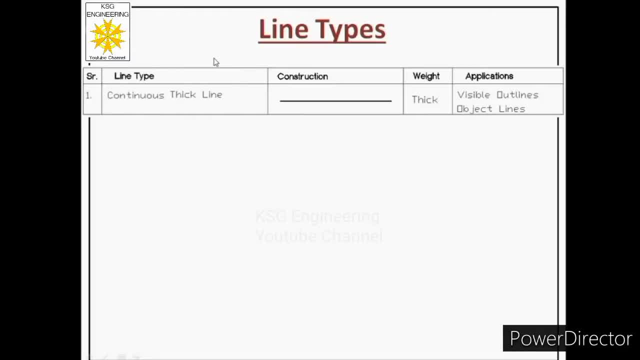 Similarly, if we want to draw a thick line, then we have to take thickness of thin line 3 times the thickness of thin line taken by us. Similarly, if we want to draw a thick line, then we have to take thickness of thin line 3 times the thickness of thin line taken by us. 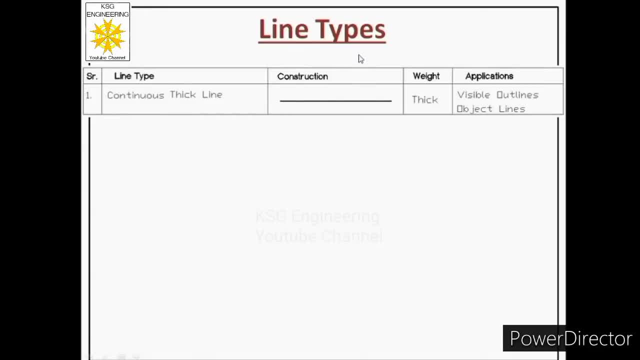 Similarly, if we want to draw a thick line, then we have to take thickness of thin line 3 times the thickness of thin line taken by us. Similarly, if we want to draw a thick line, then we have to take thickness of thin line 3 times the thickness of thin line taken by us. 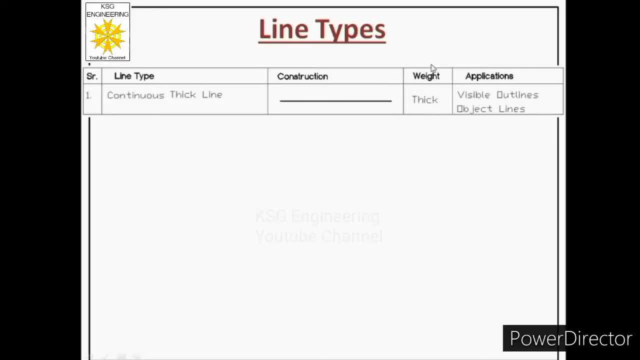 Similarly, if we want to draw a thick line, then we have to take thickness of thin line 3 times the thickness of thin line taken by us. Similarly, if we want to draw a thick line, then we have to take thickness of thin line 3 times the thickness of thin line taken by us. 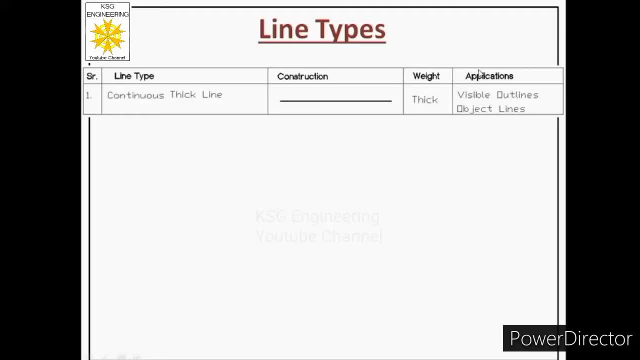 Similarly, if we want to draw a thick line, then we have to take thickness of thin line 3 times the thickness of thin line taken by us. Similarly, if we want to draw a thick line, then we have to take thickness of thin line 3 times the thickness of thin line taken by us. 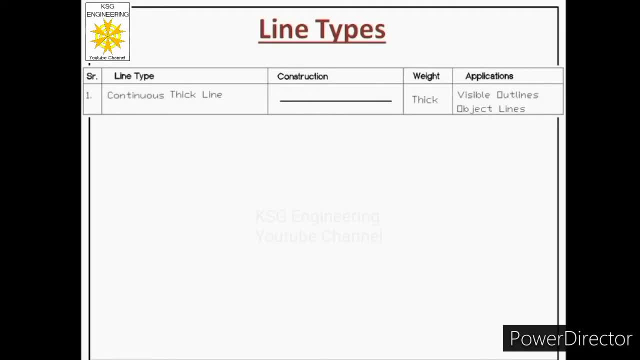 Similarly, if we want to draw a thick line, then we have to take thickness of thin line 3 times the thickness of thin line taken by us. Similarly, if we want to draw a thick line, then we have to take thickness of thin line 3 times the thickness of thin line taken by us. 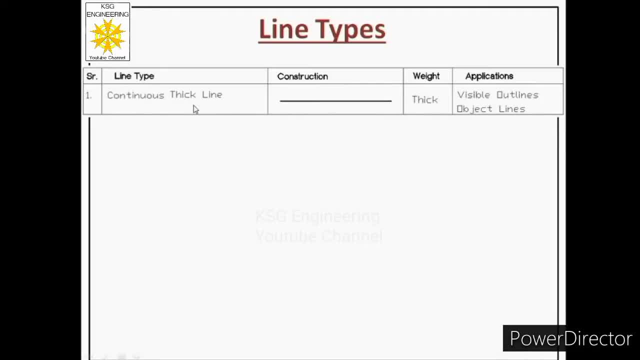 Similarly, if we want to draw a thick line, then we have to take thickness of thin line 3 times the thickness of thin line taken by us. Similarly, if we want to draw a thick line, then we have to take thickness of thin line 3 times the thickness of thin line taken by us. 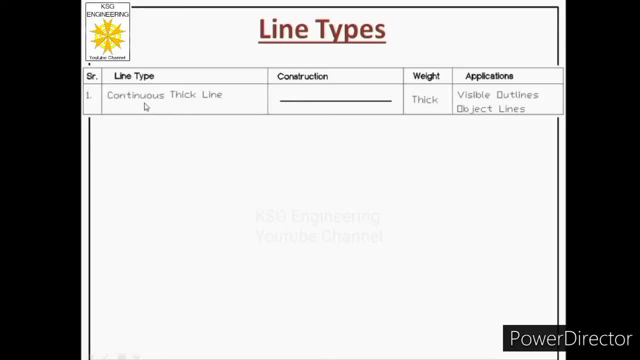 Similarly, if we want to draw a thick line, then we have to take thickness of thin line 3 times the thickness of thin line taken by us. Similarly, if we want to draw a thick line, then we have to take thickness of thin line 3 times the thickness of thin line taken by us. 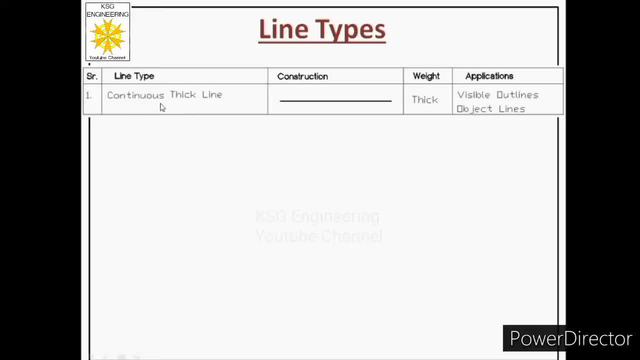 Similarly, if we want to draw a thick line, then we have to take thickness of thin line 3 times the thickness of thin line taken by us. Similarly, if we want to draw a thick line, then we have to take thickness of thin line 3 times the thickness of thin line taken by us. 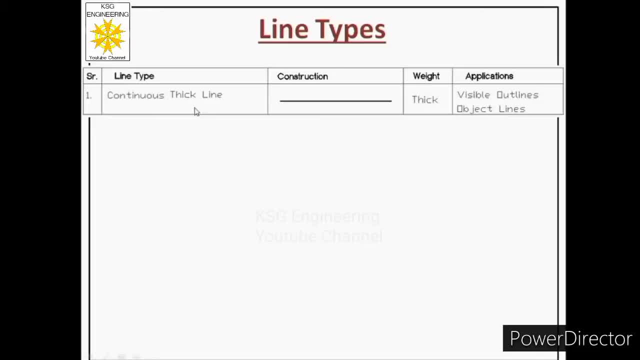 Similarly, if we want to draw a thick line, then we have to take thickness of thin line 3 times the thickness of thin line taken by us. Similarly, if we want to draw a thick line, then we have to take thickness of thin line 3 times the thickness of thin line taken by us. 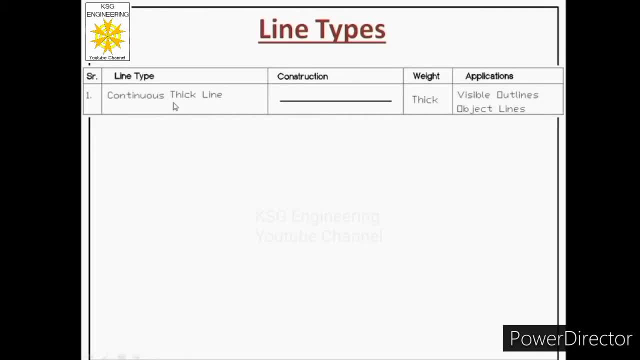 Similarly, if we want to draw a thick line, then we have to take thickness of thin line 3 times the thickness of thin line taken by us. Similarly, if we want to draw a thick line, then we have to take thickness of thin line 3 times the thickness of thin line taken by us. 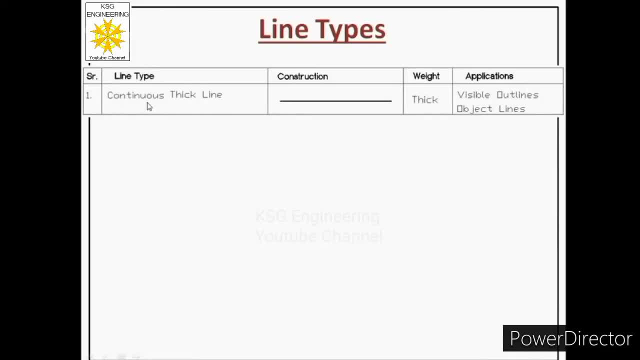 Similarly, if we want to draw a thick line, then we have to take thickness of thin line 3 times the thickness of thin line taken by us. Similarly, if we want to draw a thick line, then we have to take thickness of thin line 3 times the thickness of thin line taken by us. 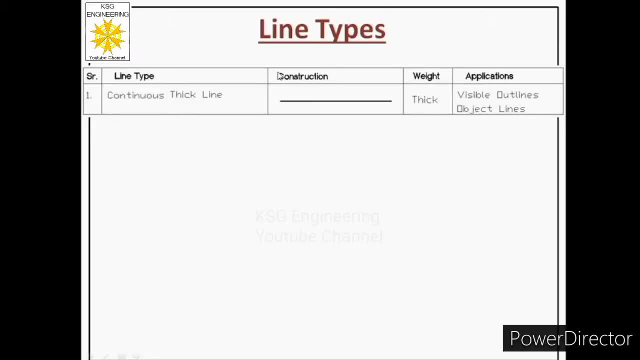 Similarly, if we want to draw a thick line, then we have to take thickness of thin line 3 times the thickness of thin line taken by us. Similarly, if we want to draw a thick line, then we have to take thickness of thin line 3 times the thickness of thin line taken by us. 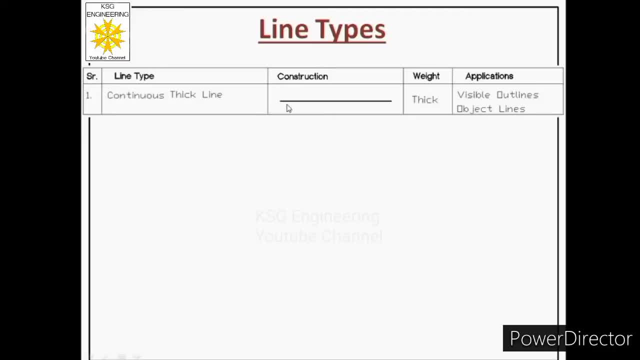 Similarly, if we want to draw a thick line, then we have to take thickness of thin line 3 times the thickness of thin line taken by us. Similarly, if we want to draw a thick line, then we have to take thickness of thin line 3 times the thickness of thin line taken by us. 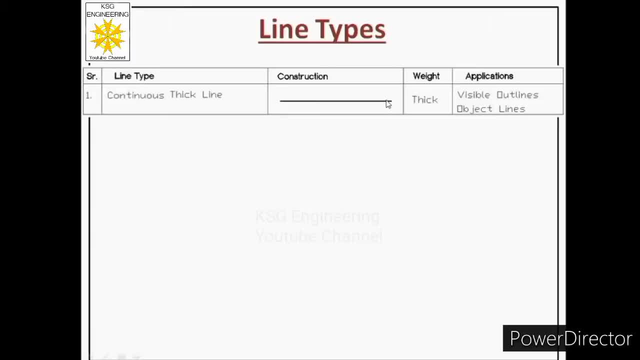 Similarly, if we want to draw a thick line, then we have to take thickness of thin line 3 times the thickness of thin line taken by us. Similarly, if we want to draw a thick line, then we have to take thickness of thin line 3 times the thickness of thin line taken by us. 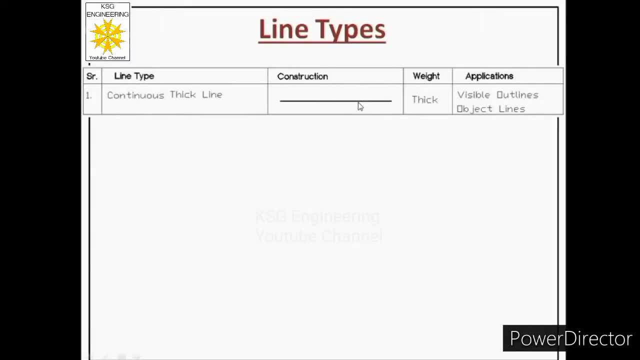 Similarly, if we want to draw a thick line, then we have to take thickness of thin line 3 times the thickness of thin line taken by us. Similarly, if we want to draw a thick line, then we have to take thickness of thin line 3 times the thickness of thin line taken by us. 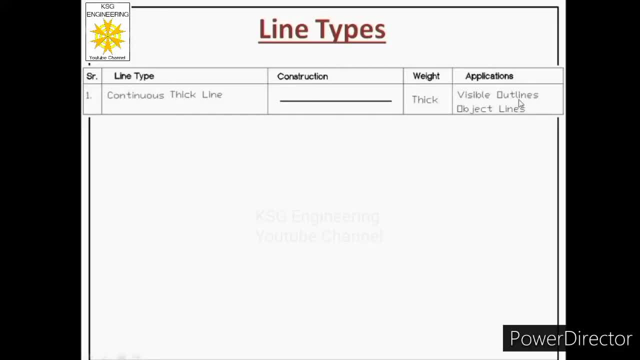 Similarly, if we want to draw a thick line, then we have to take thickness of thin line 3 times the thickness of thin line taken by us. Similarly, if we want to draw a thick line, then we have to take thickness of thin line 3 times the thickness of thin line taken by us. 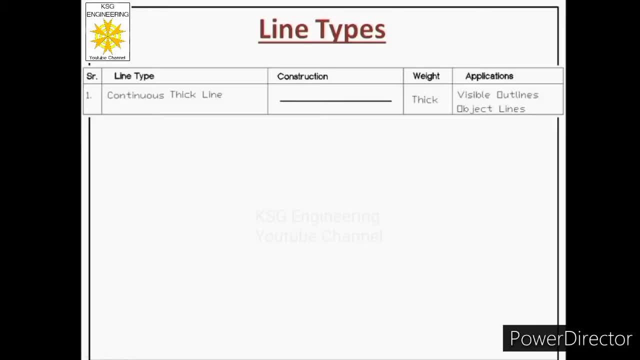 Similarly, if we want to draw a thick line, then we have to take thickness of thin line 3 times the thickness of thin line taken by us. Similarly, if we want to draw a thick line, then we have to take thickness of thin line 3 times the thickness of thin line taken by us. 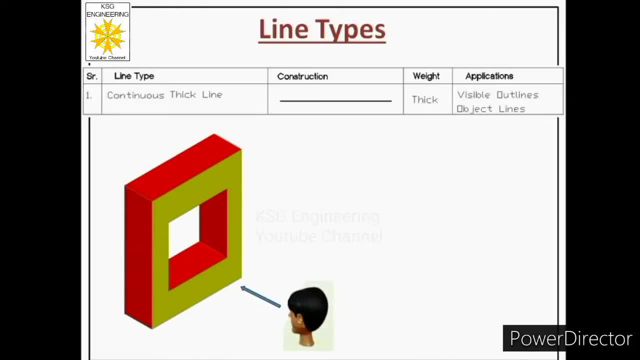 So let us understand this through an example. Suppose we have to draw front view of this object. From front side, only one face is visible, marked with yellow colour, in this object. This face is represented by 8 edges, as shown, And these edges are visible from front side. 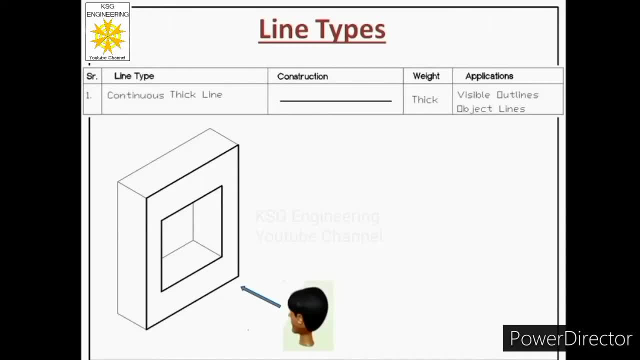 So, in order to draw the front view of this object, So in order to draw the front view of this object, So in order to draw the front view of this object, edges will be drawn with continuous thick lines, as shown over here. So we 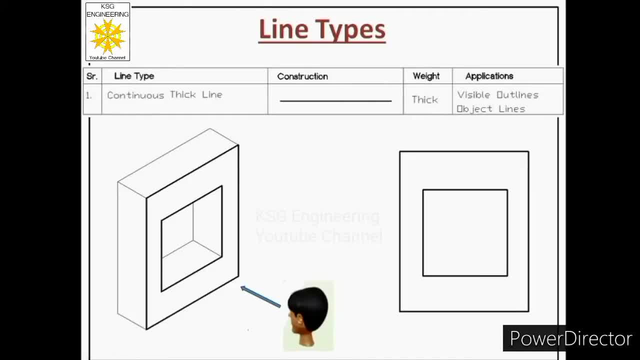 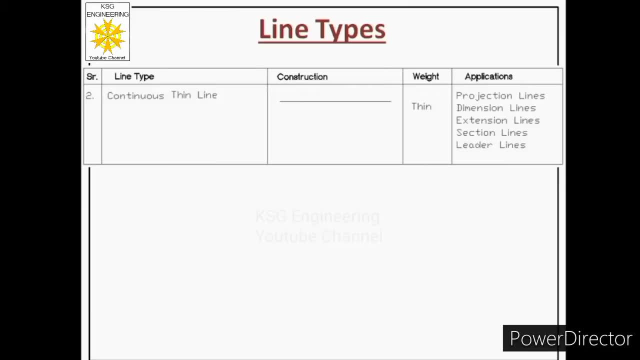 have learned that every edge or surface that is visible must be represented by continuous thick lines in the drawing. Next we will talk about continuous thin line. So construction over here is continuous and its weight is thin. So over here its construction is shown. You can see right from start to end. there is no 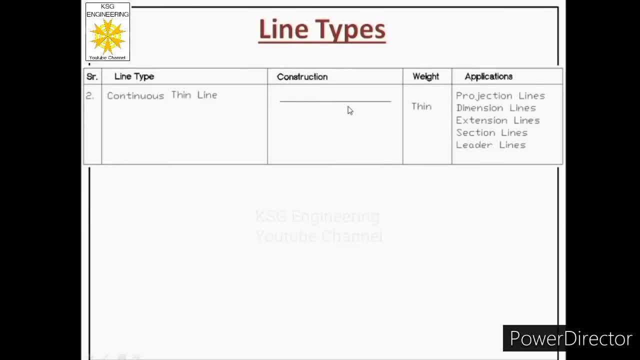 break in it. That's why we are calling its construction as continuous. but its thickness is thin. This line type is used for different purposes in the drawing. It is used to draw projection lines, dimension lines, extension lines, section lines and leader lines. So one thing we have to keep in our mind: that, in order 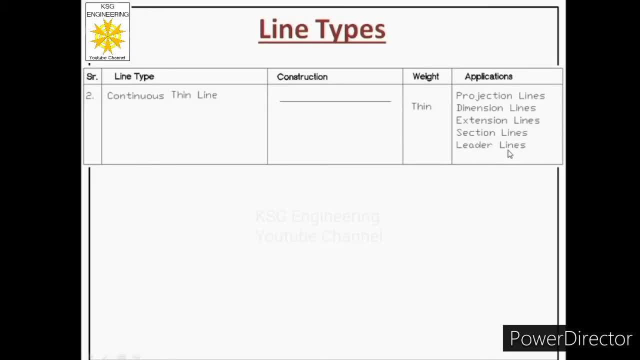 to draw such a construction. we have to keep in mind that, in order to draw such type of lines, we have to always use continuous thin line. Now let us quickly see these applications. Let us first talk about projection line. So over here front. 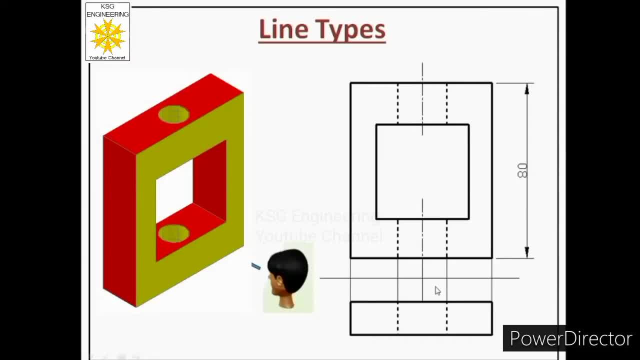 view and top view of this object are shown In. between these two views, that is, front view and top view, few lines are drawn. You can see over here. These lines are called projection lines. So the purpose of these lines is to transfer the projection of all the points of the front view. 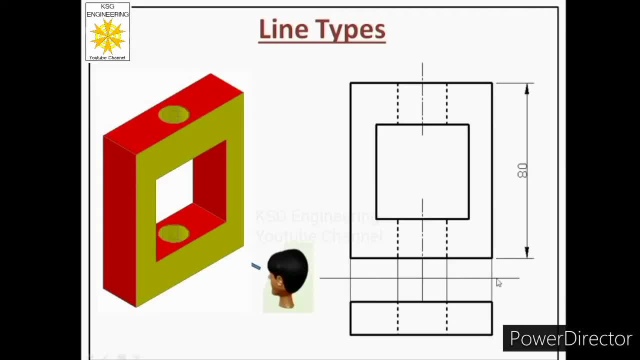 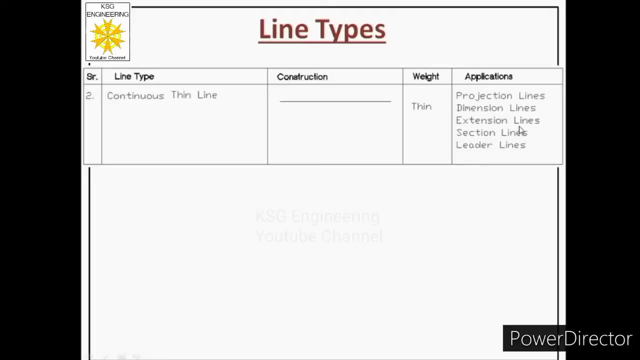 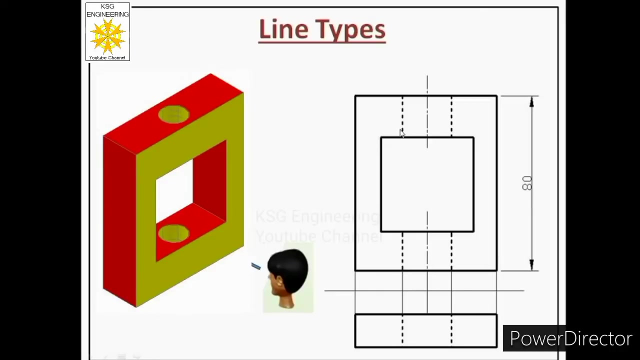 which in turn helps us to draw the top view. So whenever we have to draw these projection lines, we have to take the help of continuous thin line. Next applications are dimension lines and extension lines. Let us understand this application through an example. After drawing different views of an object, we convey the size through dimensioning. 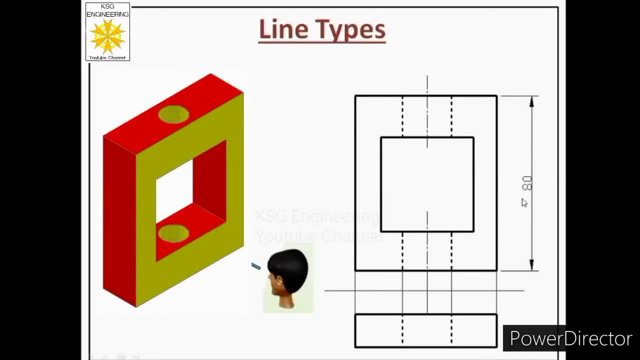 Over. here you can see. height of the object is shown, which is 80 mm. In order to place any dimension, we use two types of lines: extension lines and dimension lines. These lines are shown here, So whenever we have to draw these two lines during dimensioning. 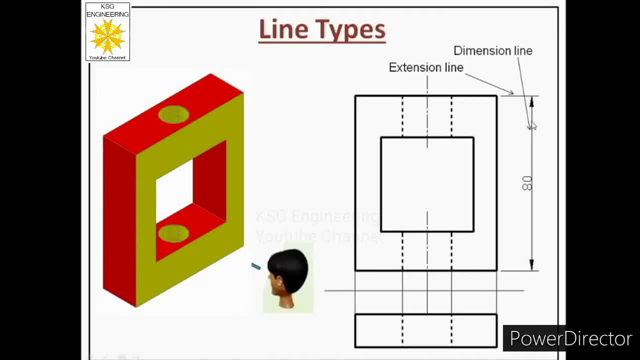 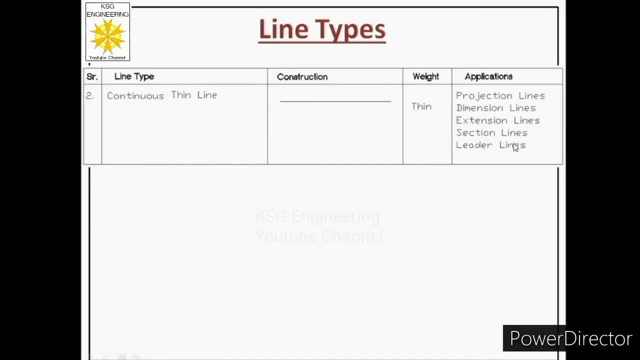 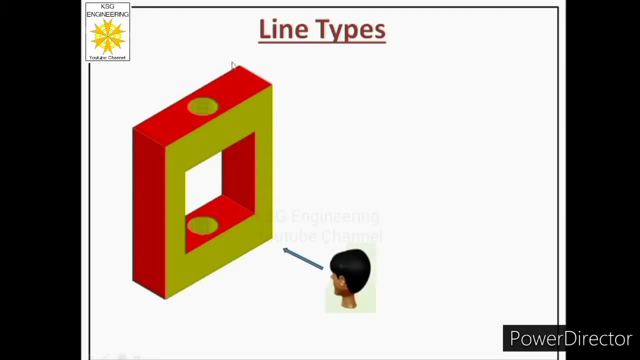 we have to take the help of continuous thin line, So we have to draw these two lines as continuous thin lines. Next application is section lines. So let us see what are section lines. Over here, an object is shown with two holes, One at the top and the second one is at the bottom side. 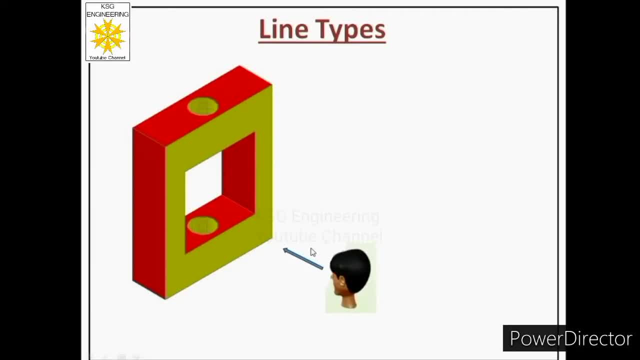 These holes are not visible from front. So in order to show internal detail more clearly, we use one method called as sectioning. This method you will learn in the coming lectures, But over here, in order to understand section lines, I will give you the brief of that method. 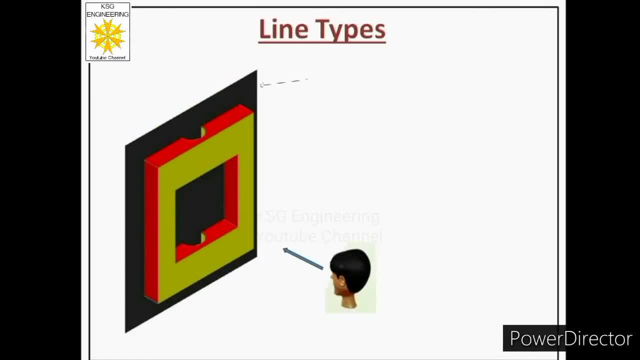 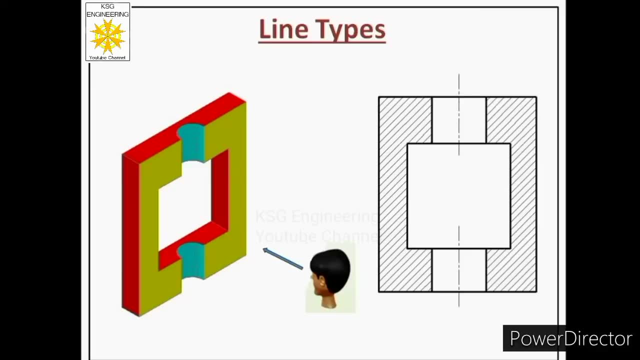 So in sectioning process we use to cut the object from a particular section with an imaginary cutting plane which removes front half of the object to show the internal detail. The views so obtained are called section views, And in these views we can see that 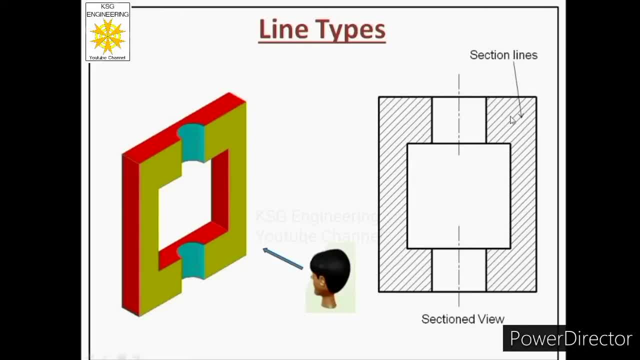 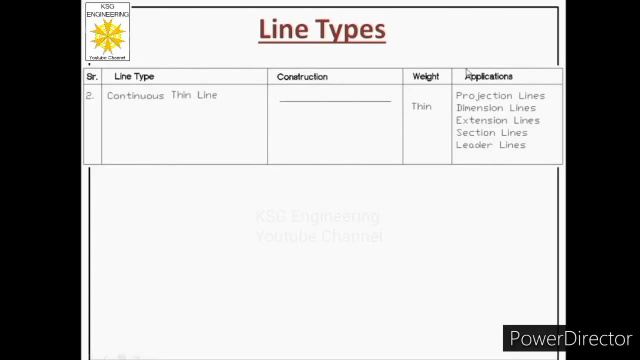 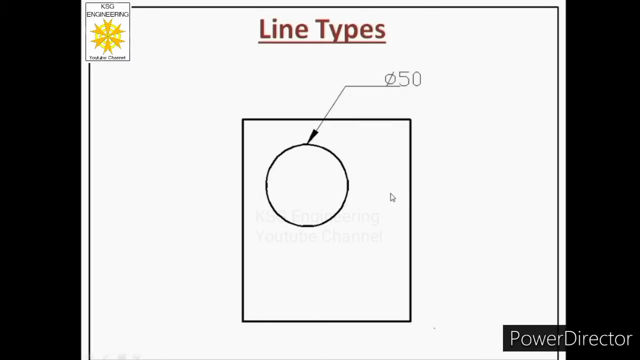 we place section lines, which represents the cut area of the object. So whenever we have to draw section lines in the section view, we will use continuous thin lines. The next application of this line is leader line. In dimensioning chapter you will learn about the use of leader lines in detail. 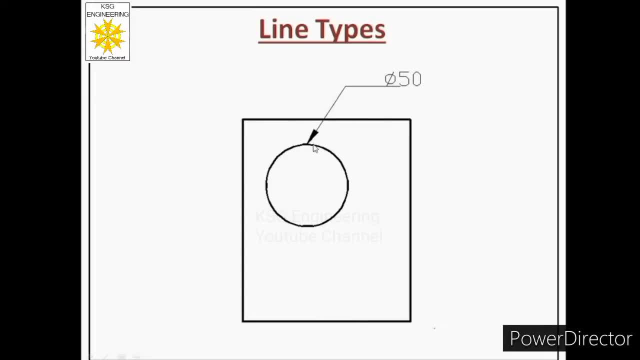 Basically, it consists of an inclined line with an arrowhead at one end which points towards a particular entity in the drawing, and a tail on the other end on which some information is given about that entity. So if we have to draw a leader during dimensioning, 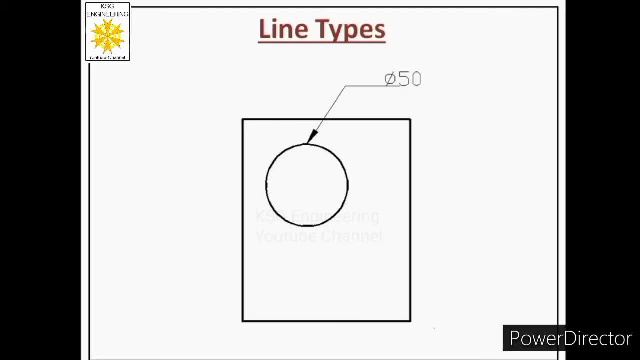 we have to draw it with continuous thin line. Next we will talk about dashed medium line. For this line, construction is dashed and its weight is medium. It is used to represent hidden portion of the object in the drawings. Let us understand this through an example. 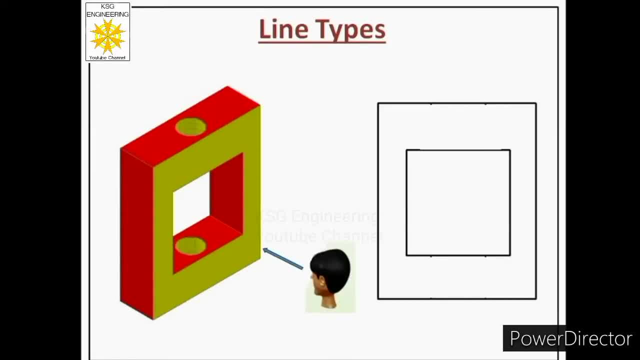 Suppose we are given this object and we have to draw its front view. As you can see, the two holes shown in the object are not visible from front. So in order to represent these holes in the front view, dashed medium lines are used. 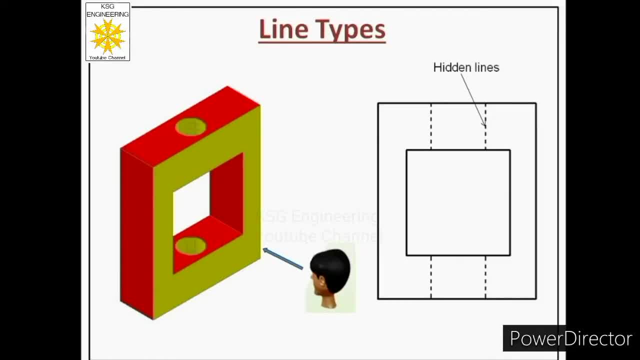 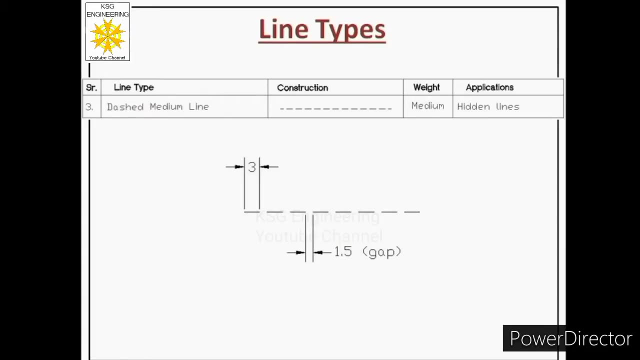 So in other words, we can say that if dashed medium lines are drawn in the drawing, then we must understand that that particular area of the drawing is not visible from front side. Its construction is very important. In order to draw this line, we have to draw small dashes of 3 mm length, separated by 1.5 mm gap. 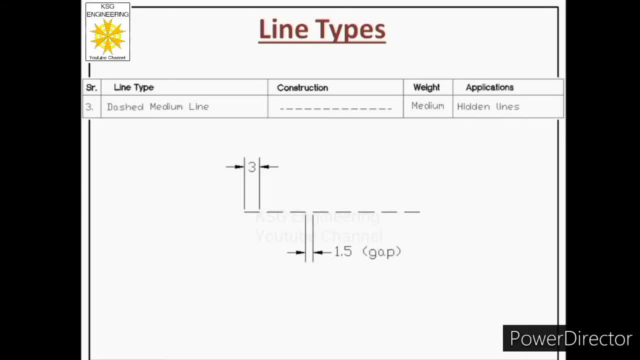 This pattern we have to draw up to required length. Next we will talk about chain thin line Construction, for this line is chain and its weight is thin. It is used to represent center lines. Let us understand this through an example. Suppose we are given this object and this is its front view. 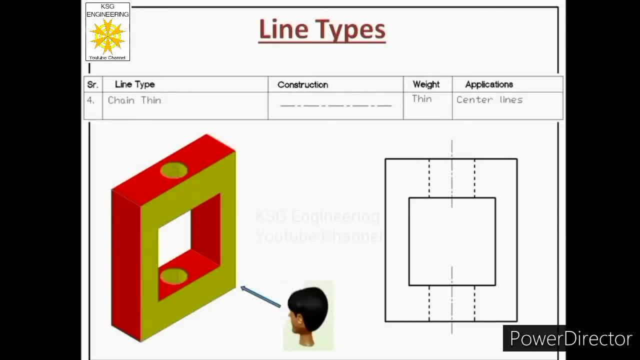 Now you can see in the front view the axis of both the holes or the center lines are drawn as chain thin lines. These lines are used to indicate axis of symmetrical parts or axis of symmetry of the object. Let us see its construction in detail. 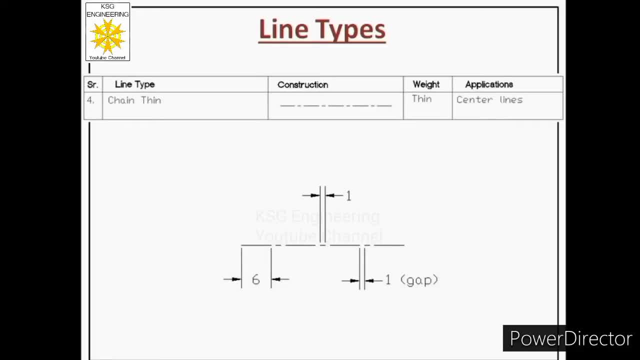 It is a chain of long and short dashes. The length of long dash can be drawn either 10 mm or 6 mm, But the length of short dashes will remain the same: 1 mm. in both the cases, These dashes are separated by a gap of 1 mm, as shown in this figure. 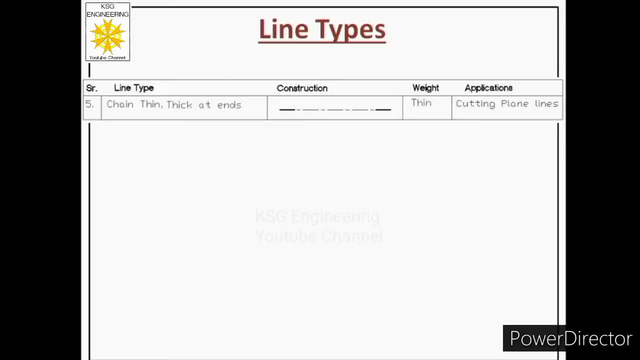 The next line type is chain thin, thick at ends. Construction over here is chain and its weight is thin and thick at ends. It is used to represent cutting plane lines. Let us see its construction first. Its construction is similar to chain thin. That means it consists of long and short dashes. 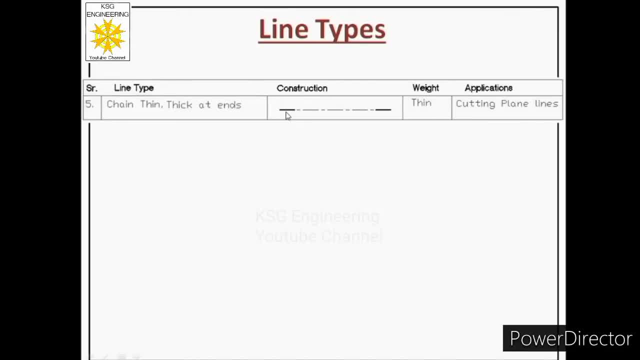 So the length of long dash we can take as 10 mm or 6 mm, But the length of short dashes will remain as 1 mm And the gap between any two dashes will be 1 mm, Like we are taking in chain thin line.